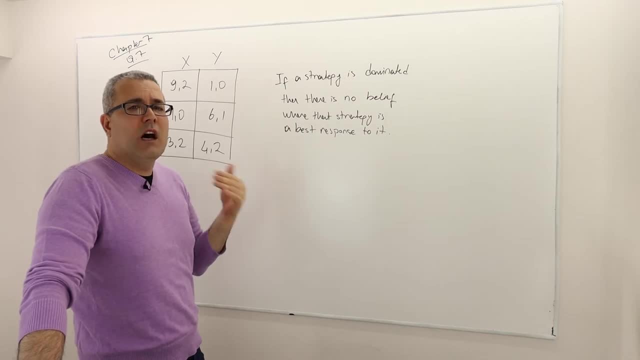 going to write the formal definition, but intuitively, a dominated strategy means, guys, there is another strategy of this player, all right, where that strategy always gives a higher, strictly higher payoff, all right. so always means- I keep underlying this- but always means whatever the opponents there might be. 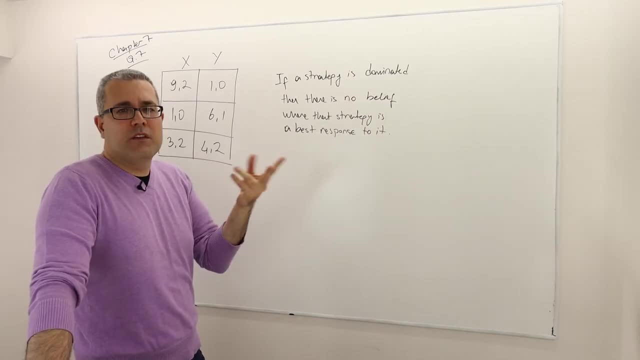 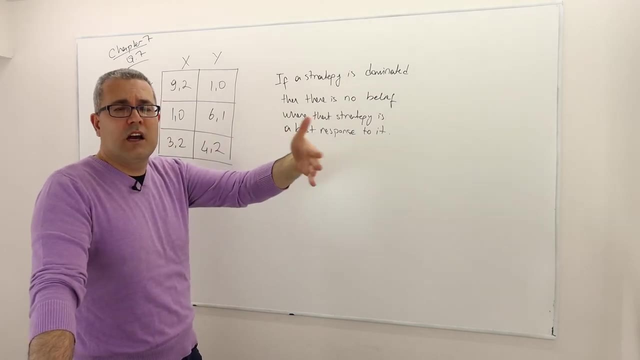 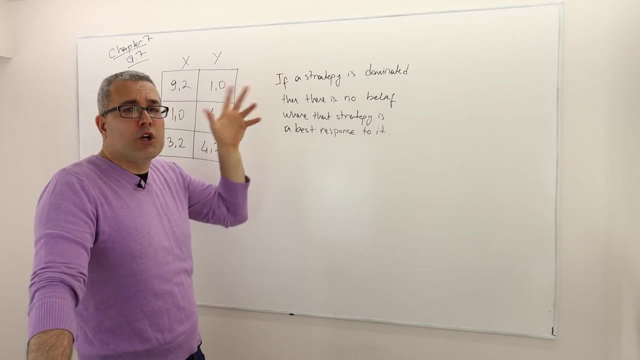 more than one opponent in this game. so if, for example, there are three players, and I'm talking about Player 1, his opponents are Player 2 & 3, right? so regardless of what the other guys, what the opponents do, all right. well then, the playing that strategy should be worse than the other strategy. if my strategy 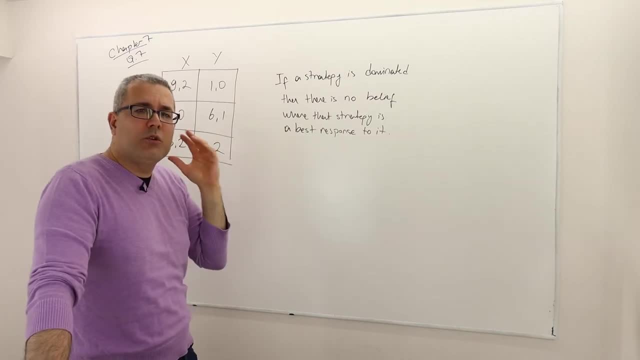 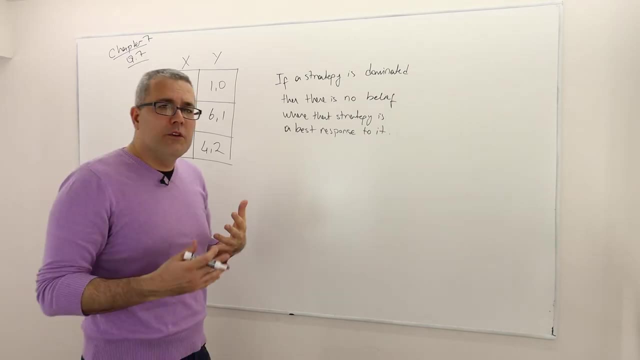 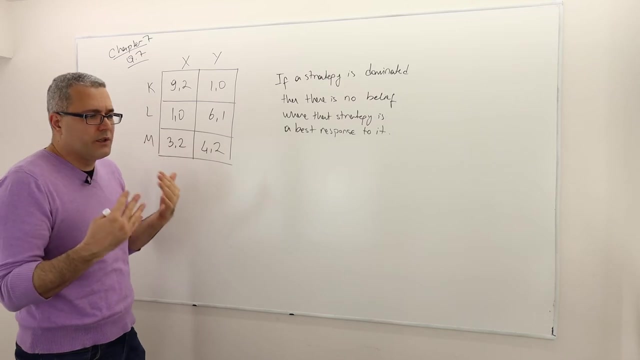 strategies dominated, all right. So again, conceptually and intuitively, a dominated strategy means inferior strategy. There is something better, all right. But obviously when you sort of do it in practice, you have to be careful about it. all right, I know you. 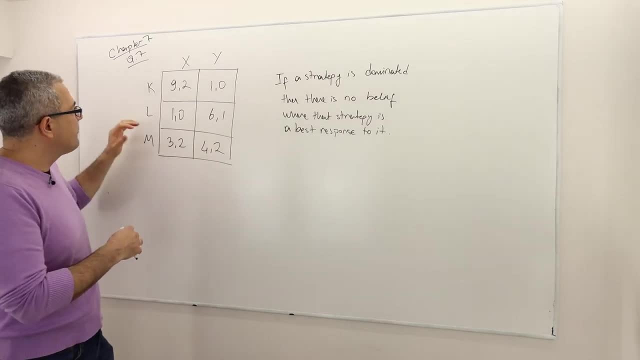 understand this intuition, but when it comes to applying it, for example, is there any strategy here? Let's look at pure strategies. all right, Meaning for player one, there are two pure strategies other than M, K and L, right, So if M is dominated, it should be either K or L. But 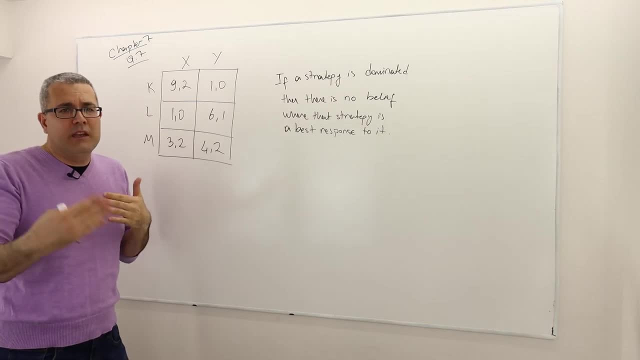 don't forget, sometimes pure strategy does not dominate a pure strategy. So we also need to look at mixed strategy. But here let's first focus on the pures. So here, K, does this dominate M? I mean, is it really always better? No, it's not always better. For example, K is better than M. 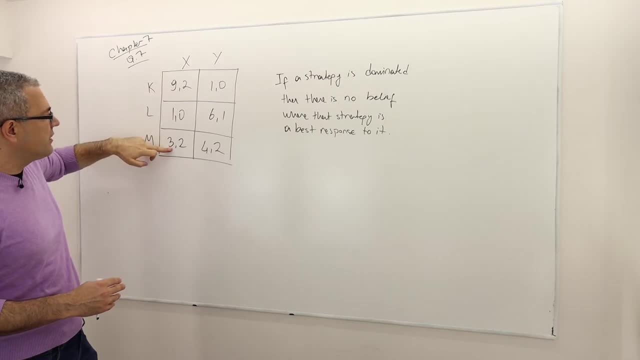 when the second guy is playing, So here K is better than M. when the second guy is playing X, right, Because nine is higher than three. But when the second guy plays Y, so one is worse than four. So therefore I look at column Y, So every column, one strategy should be giving strictly. 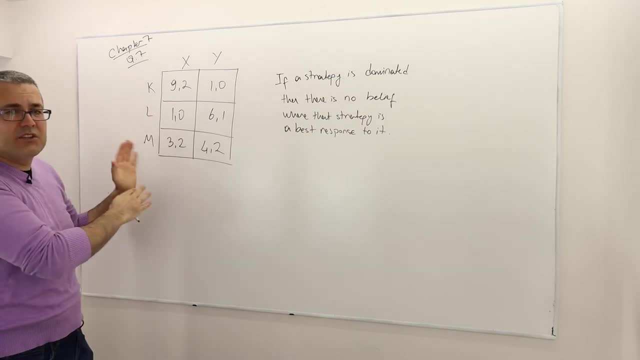 higher payoff than the other payoff- all right- Than the other strategy. I'm sorry, So here we don't have this. So K does not dominate M. Similarly, L does not dominate M, because it's sometimes better, yes, but sometimes worse. 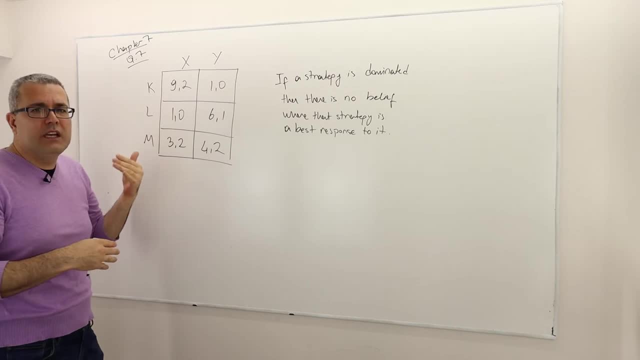 Or sometimes equal, maybe all right. So if sometimes they're equal, for example, if this was three rather than one, we still couldn't say L is strictly dominating. M right, It's not strict domination, It's what we call weak domination. But we're not really into the concept of weak. 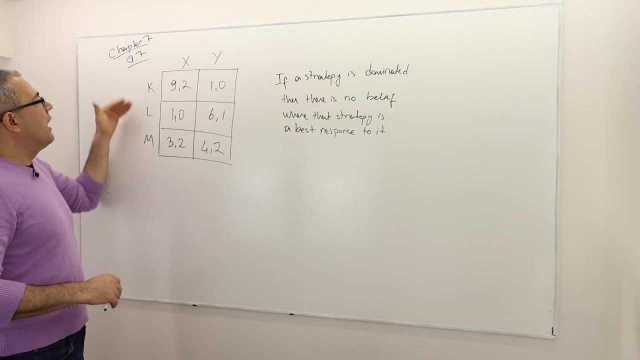 domination. So that means for player one, there is no pure strategy that's dominating M. Well, but is there any mixed strategy that dominates M? I did not solve this question before this lecture, but when I look at the payoffs, my guess is that yes, there is, And I'll talk about it in a minute. But let me come back to here. 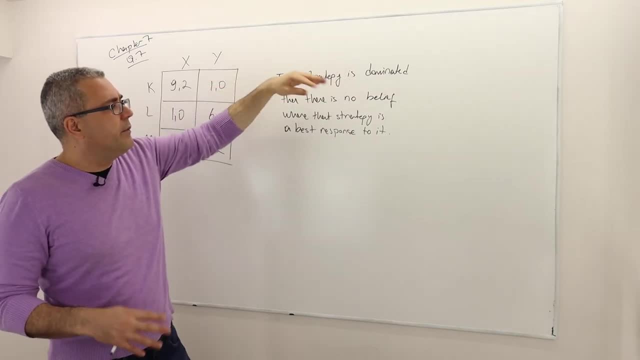 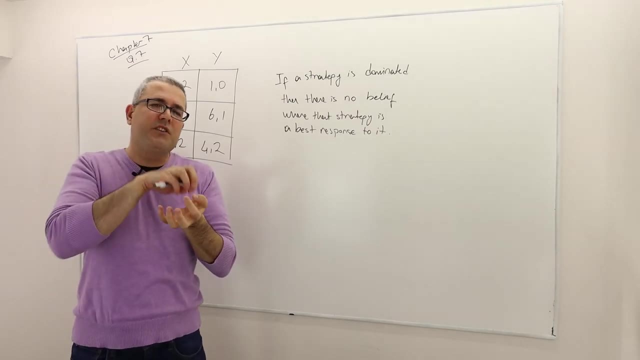 Remember I said if a strategy is dominated well, then there's going to be no belief where that strategy is a best response. So, by the way, best response is a part of this strict domination idea, But nevertheless it's a very, very important concept in this. 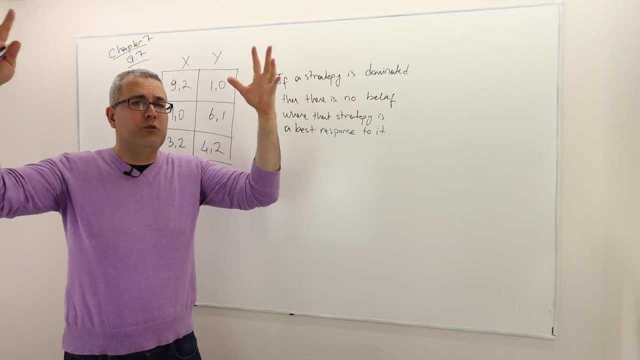 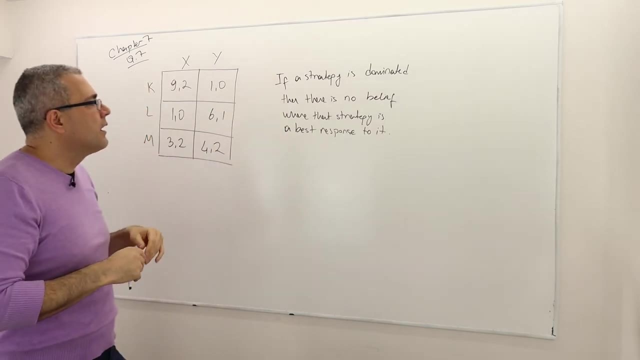 conversation, So I'm going to talk about it in a minute, So let's get started. All right, Maybe if the Nash equilibrium is the most important, second best, I'm sorry- the best response concept is the second most important concept. All right, All right, So 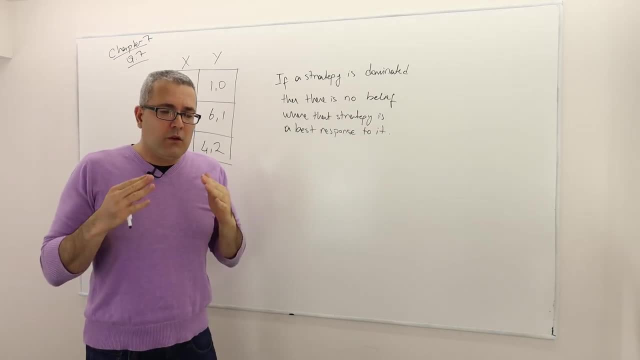 what is best response? Best response is the following: Look, this is a game environment, the strategic environment. right? My payoff depends on my opponent's strategies. So, or my beliefs about my opponent's strategies, All right. So, given my opponent's strategies, I'm going to 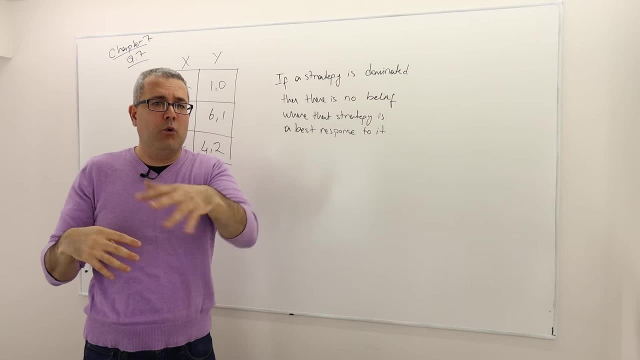 strategy, or, given my belief about my opponent's strategy, what is the best action I can pick? All right, So best action, I can pick- Well, that action. or what is the best strategy I can pick? Well, that best strategy. well, we call it as a best response strategy. All right, That's. 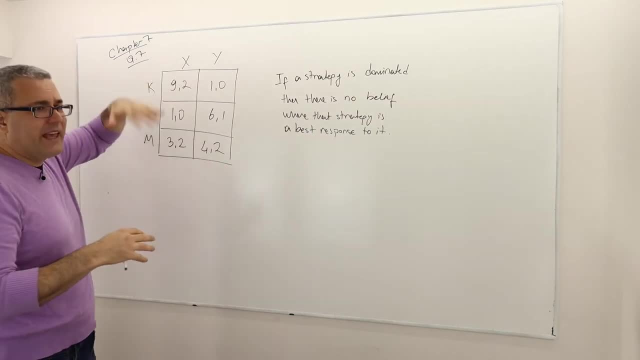 conceptually what it means. So for example- again a very simple example, I know. But let's suppose I believe my opponent is going to play X For sure, All right, So I don't have any mixed beliefs. So if my opponent is going to play X, 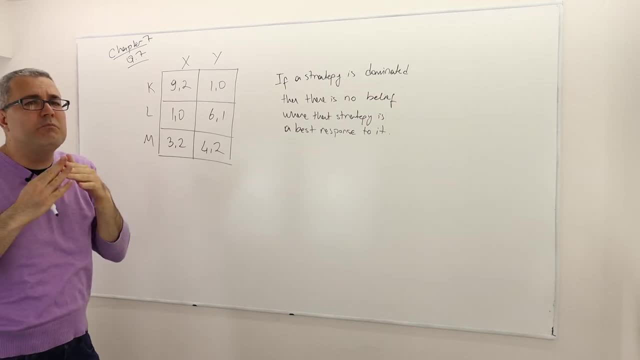 what is my best response, Meaning? what is the strategy that gives me the highest payoff? Well, is it K and get nine, Is it L and one? And is it M and three payoff? Well, obviously it's K. So K is the best response to X. All right, What about if my opponent is playing Y? Well, 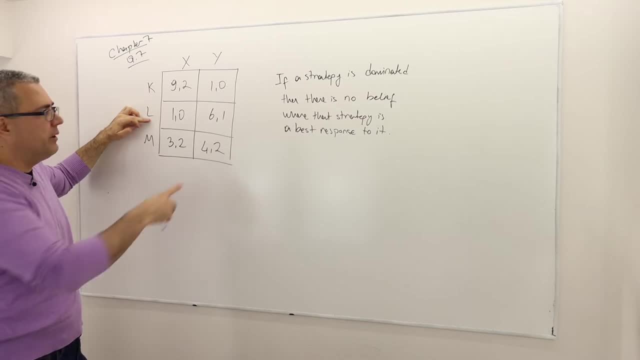 if my opponent is playing Y, my best response is L, because six is the highest payoff. All right, So what I do observe in this game is that, well, K and L, they both are best response to some belief about my opponent's strategy. Pure beliefs, but some beliefs, Well, here. 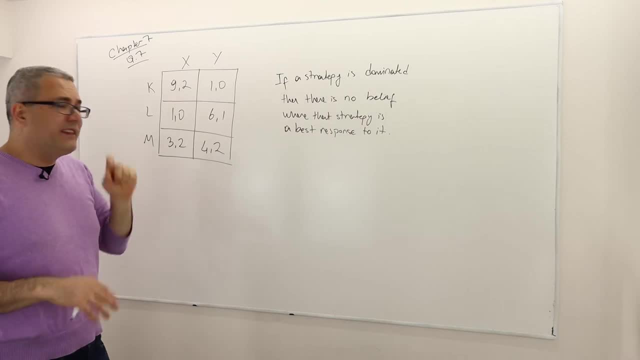 M is never a best response to any pure strategy. That doesn't mean that M is a strictly dominated strategy, Because, again, I did not look at mixed beliefs. What if my opponent plays X? What if my X and Y say half and half probability? Well then, maybe M is going to be a best response. I don't. 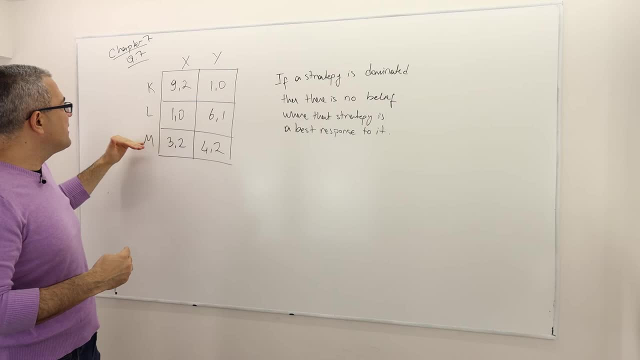 know this yet because I didn't check. But you know what? If a strategy is not a best response to any pure strategy, well, trust me, it's a good candidate. Candidate, though right, It's not a sure thing. It's a good candidate that this strategy is, in fact, strictly dominated. All right, 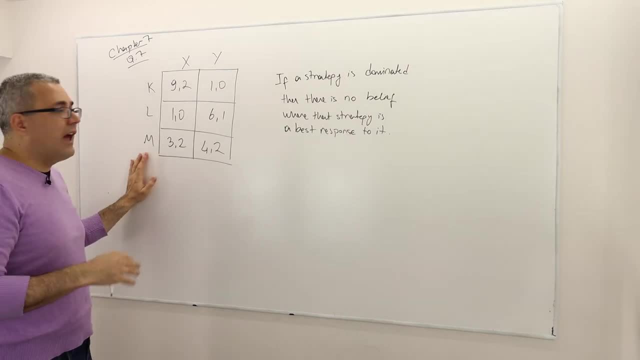 So this is sort of my hunch Reasoning behind. So it's not really hunch, It's sort of educated guess. So M probably is a strictly dominated strategy. So all I have to do is to find a mixed strategy between K and L. 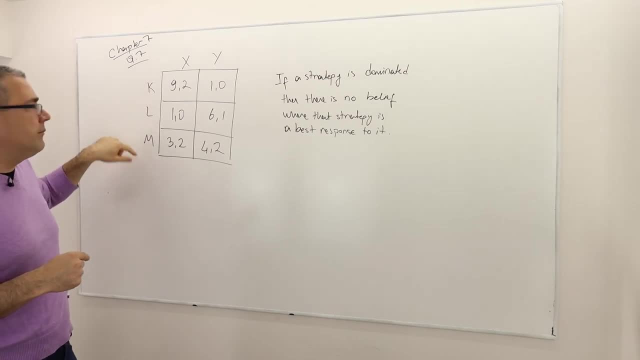 because K alone itself cannot dominate M, L alone cannot dominate M. But maybe a mix of K and L, right, Because here nine and one. when I mix them it may end up something higher than three, Although by itself L cannot be higher than three. And again, by mixing K and L I mean mixing one. 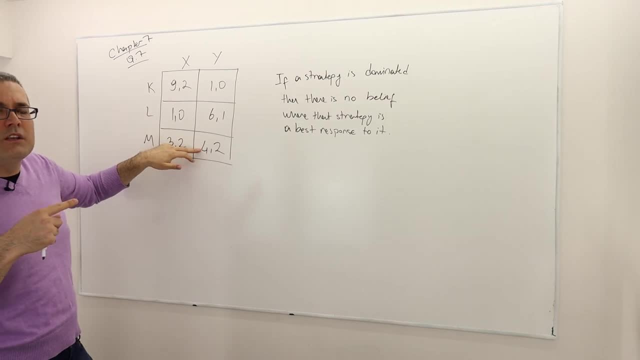 and six payoff, I can get something higher than four. So that correct mixing is very important. But if I can mix K and L well, then that may actually dominate M. So what is that mixture? And this is exactly what the question is asking. So let's call this P and this is one minus P. 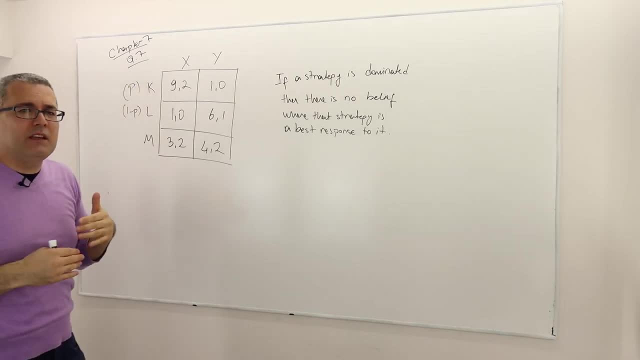 Why I put P one minus P. Well, I am mixing between these, these two strategies, All right. So there's no point of saying this is P one, this is P two, because I know P one plus P two must be equal to one. Because, once again, I am mixing between these. 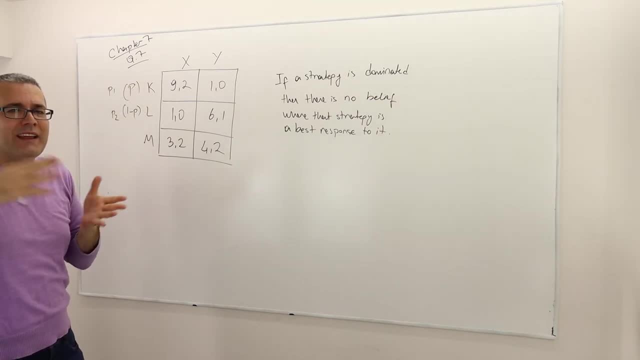 two strategies only, So the probability must add up to one always. So for that reason, I call this P and this one minus P. So what am I going to do? Well, for M to be, for M to be dominated. remember, dominated, strictly dominated means the same thing in this course. So for M to be dominated, 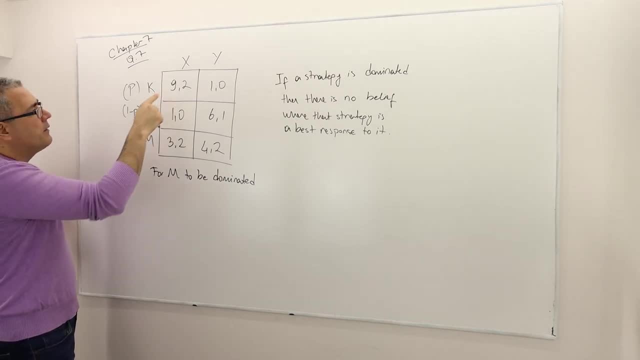 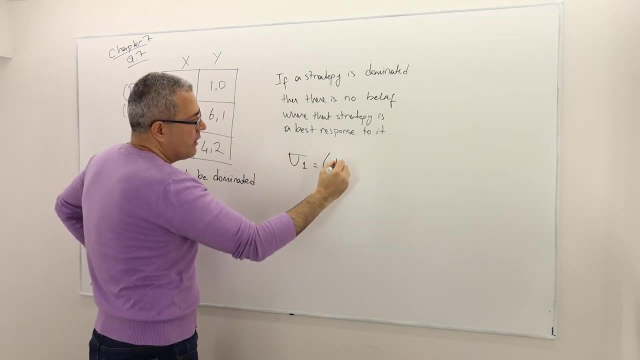 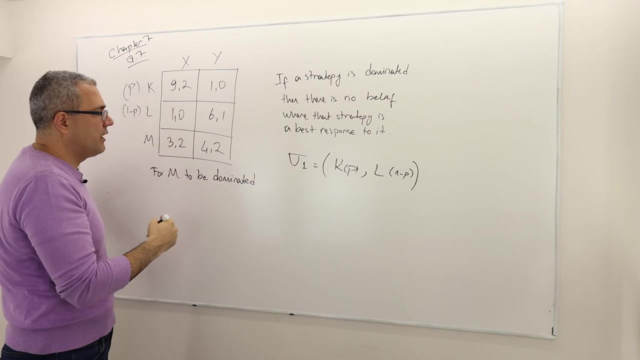 I have to have the following. First, my strategy from this mixture. So let's call this sigma one, where I play K with P probability and L with one minus P probability. Okay, That's my mixed strategy. So the expected payoff of sigma one: All right. 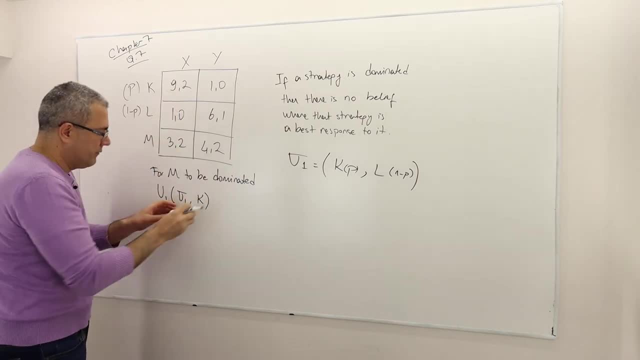 Given that my opponent is playing X. I'm sorry, I say X, but I write K. You see what I mean. Sometimes I do make such silly mistakes. So what is my expected payoff? So I am playing this sigma, one mixed, and my opponent is playing X. So what is going to be my expected payoff? Well, it's nine. 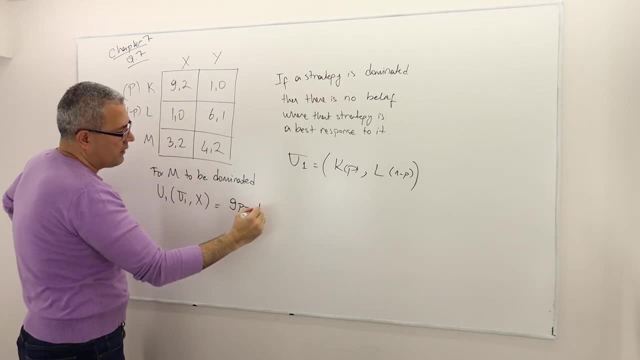 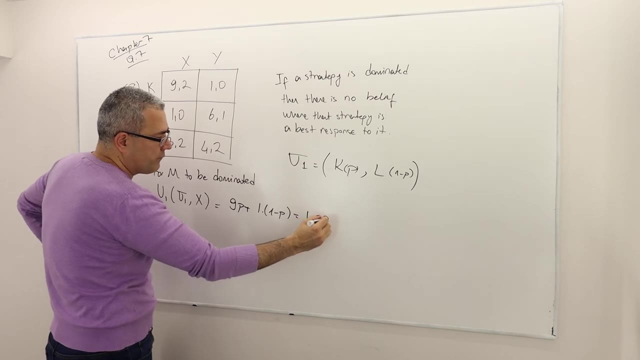 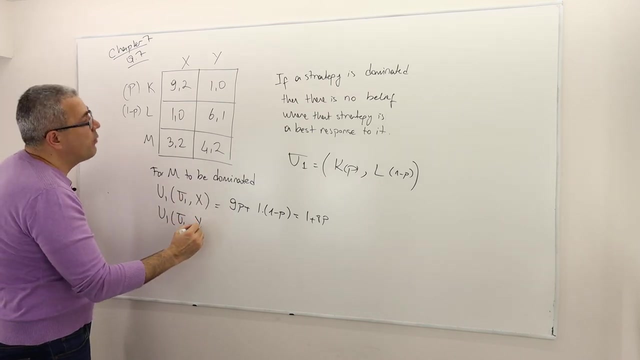 times P plus one times one minus P. So if you sum them up or simplify, it basically means one plus eight P. All right, And then what else My expected payoff if I play this mixed strategy but my opponent is playing Y? what is that? equal to? Well, that equals to. 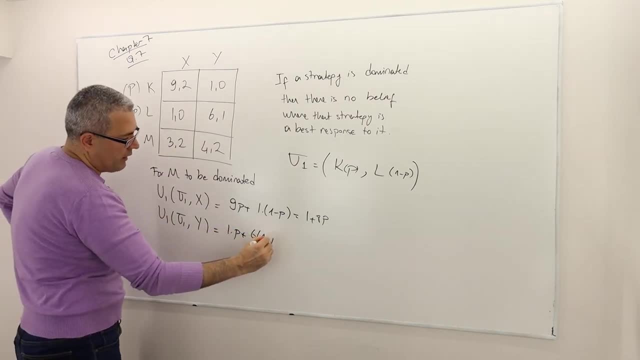 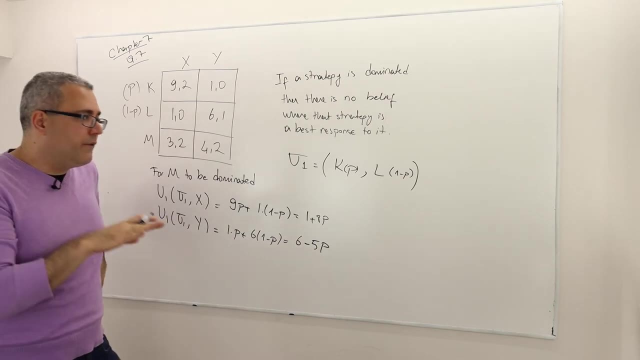 one times P plus six times one minus P. So if I add it up or simplify it, I'm going to get six minus five P, All right. So if you remember, a strict domination means there exists some sigma one. So sigma one, sigma one, sigma two, sigma three, sigma four, sigma five, sigma six sigma. 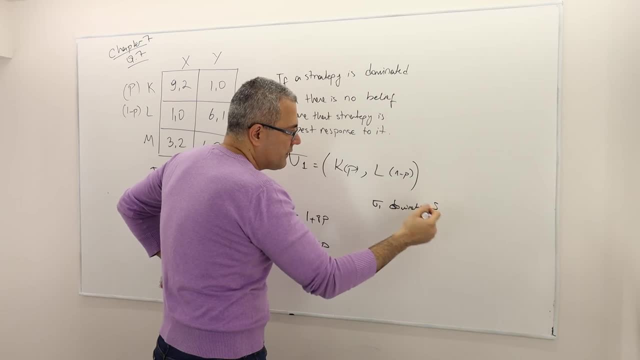 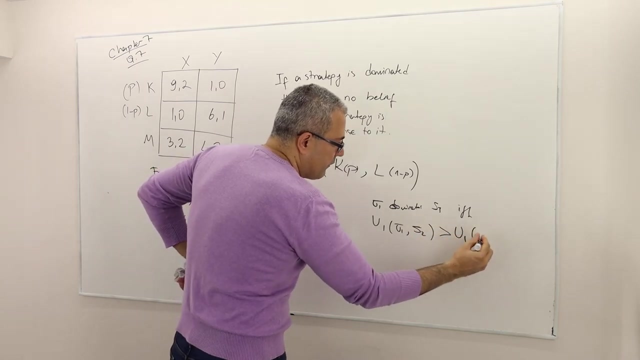 one dominates S1.. So the first player strategy: if, and only if So, the expected payoff of sigma one- let's call this S2- greater than strictly greater than expected payoff of S1, S2 for all S2.. Remember. 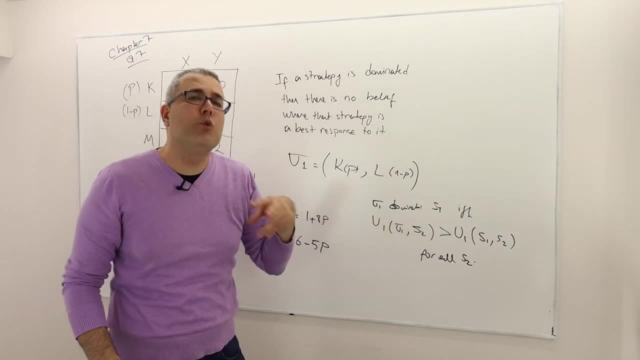 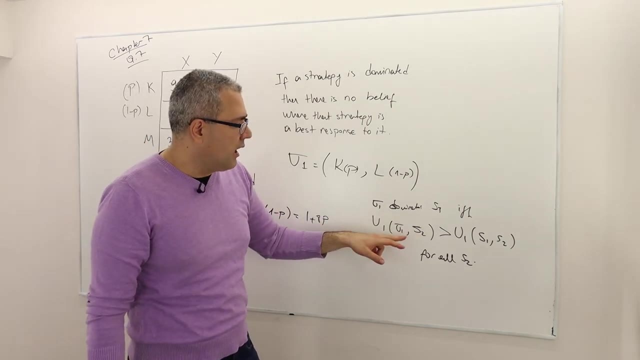 So that was the formal definition. What does that mean For every pure strategy? so go back and look at the definition For every pure strategy. go back and look at the definition For every pure strategy. my opponent follows the sigma one guy. My expected payoff of playing the sigma one guy. 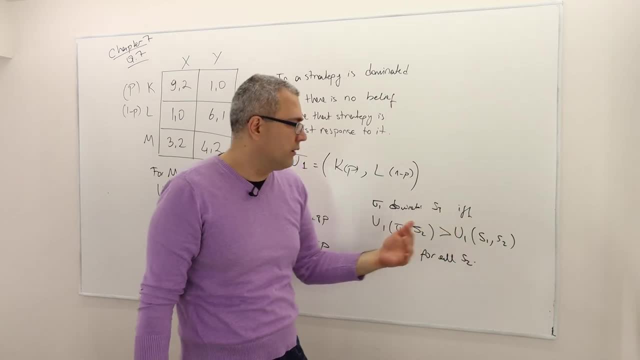 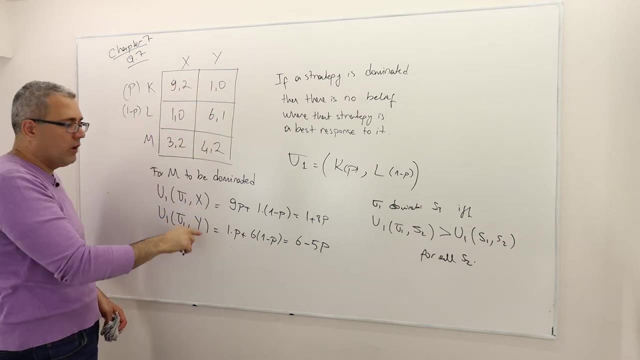 is going to be higher than my expected payoff of playing S1.. All right, So that was the idea And this is why I calculated those expected payoffs, given that my opponent plays X and Y because he has two pure strategies. So the strict domination I mean this guy will imply the following: So if 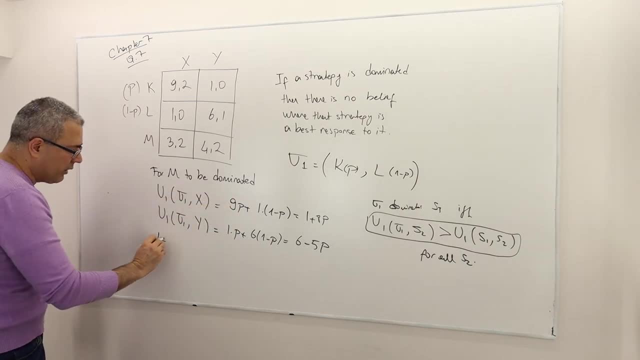 for M to be strictly dominated, I have to have the following: One plus eight P- the combination of these two must be greater than three. when I play M, All right- And one- I'm sorry, six minus five P must be greater than four. 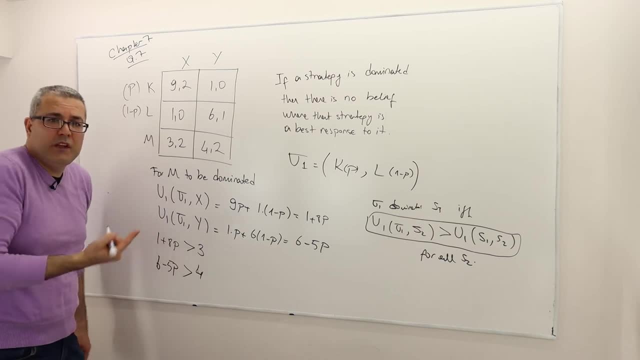 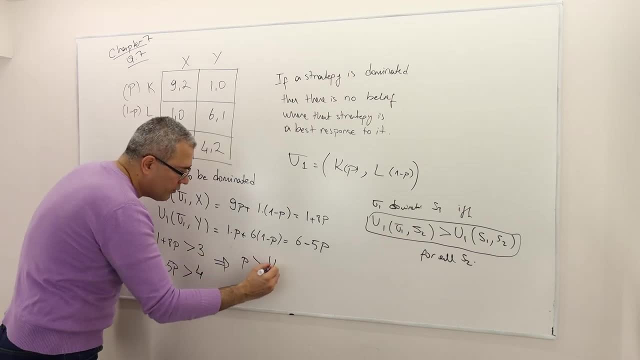 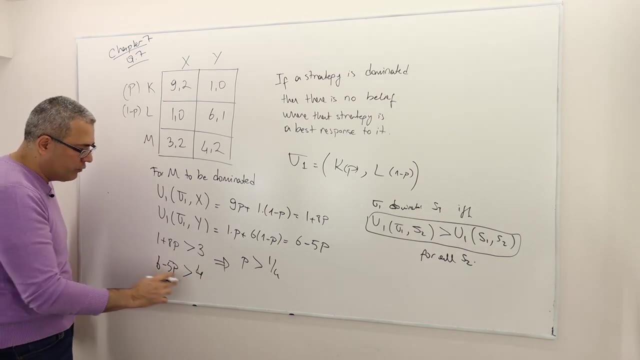 that means P is greater than two over eight, which is one over four. And the second guy means I'm going to send the five P to the other side to make it positive. So it's going to be two over five. So P is less than two over five. So that is point twenty-five, right, And that's point 20..